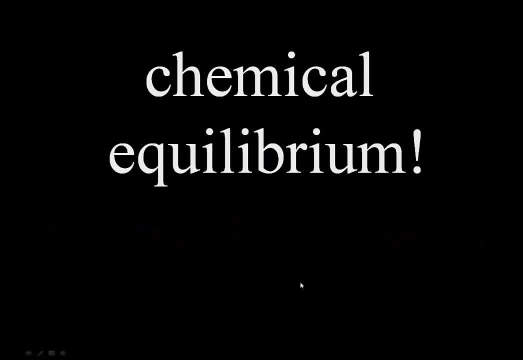 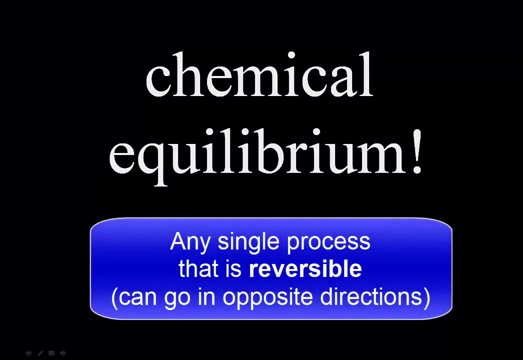 Okay, we're back today with chemical equilibrium, and I think the first place to start would be to get a working definition of what chemical equilibrium is, and from a chemistry perspective, we're looking at any process that can go in two different directions or two opposite directions. 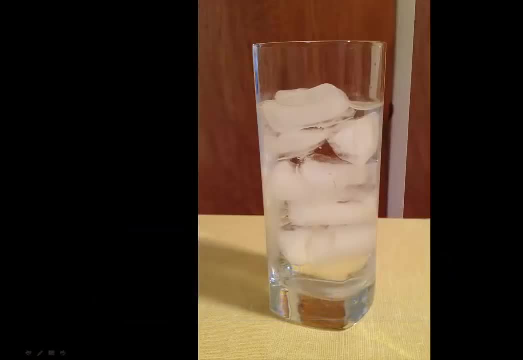 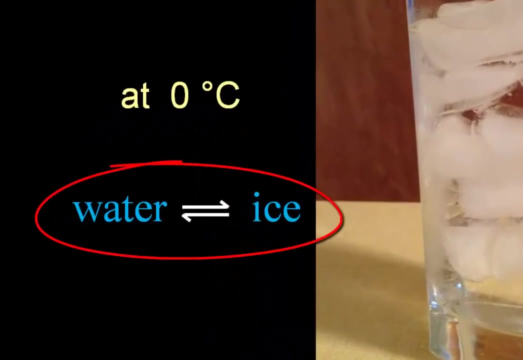 So an example of that would be water and ice. Water at zero degrees can freeze. that's the freezing point of water, and it turns into ice. but zero degrees is also the melting point of water. and so here's a single process going in both directions simultaneously, and so we could write it with a double arrow: water going to ice simultaneously, ice becoming liquid water. 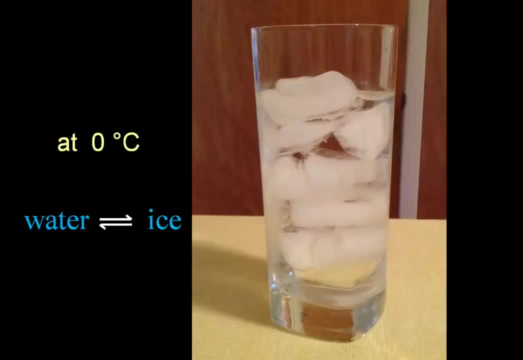 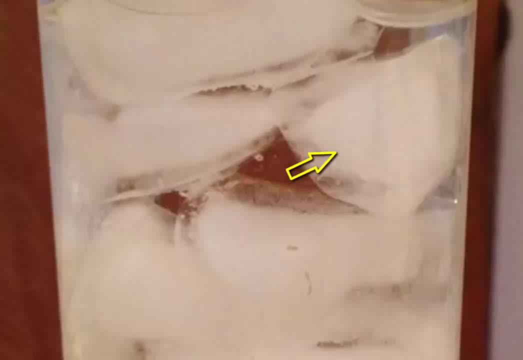 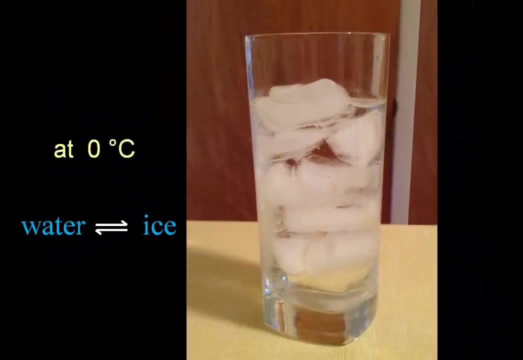 And if you have a process that can go in opposite directions, it can reach an equilibrium At zero degrees. water is simultaneously turning into ice, while ice is turning into liquid water, and if that is occurring at the same rate, which it would be at zero degrees, then we would have reached an equilibrium. 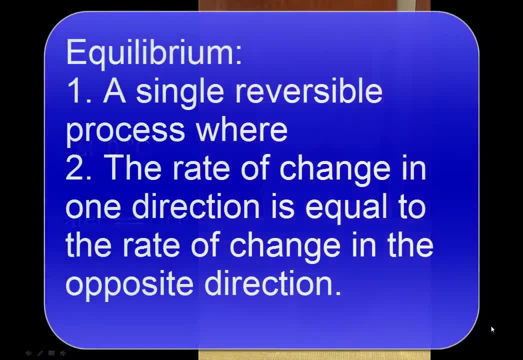 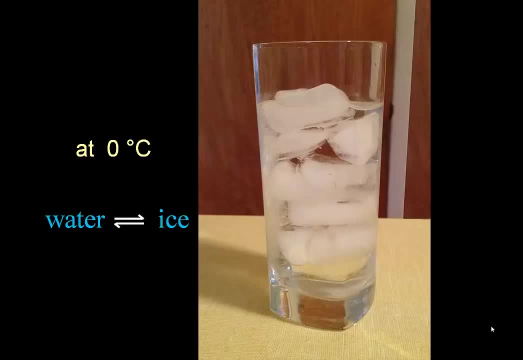 So our working definition of equilibrium can be a single process that can go in opposite directions, Where the rate of change in one direction is equal to the rate of change in the other direction. So here, at zero degrees, we can have an equilibrium where the amount of liquid water freezing into ice is equal to the amount of ice that is melting into liquid water. 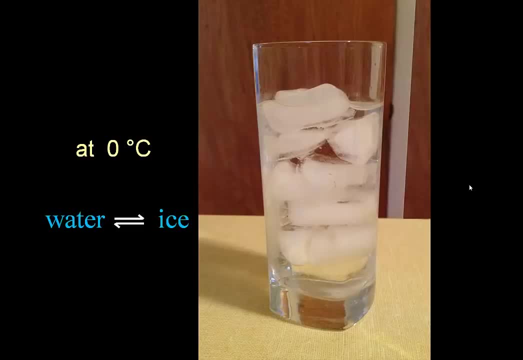 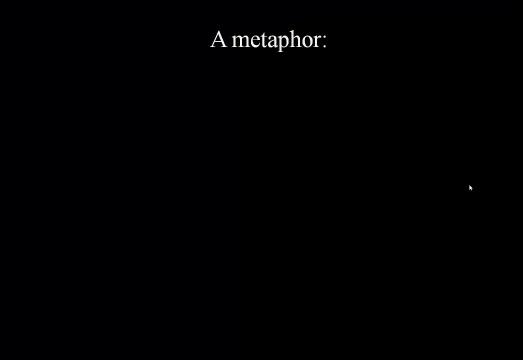 Let's now take a look at chemical reactions and what sort of chemical reaction we would be looking at that could reach an equilibrium. But to better access that idea, let's first take a look at a metaphor. Our metaphor is two floors of a store that are connected by up and down escalators. 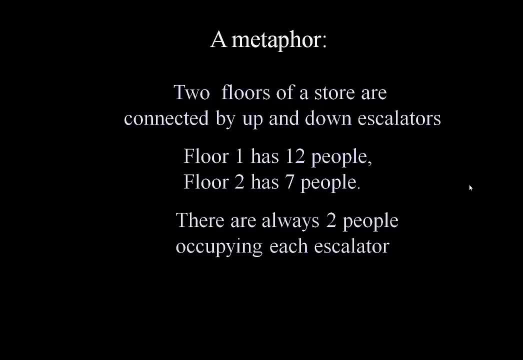 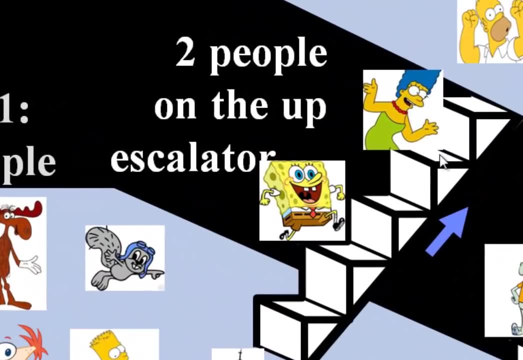 The first floor has 12 people, the second floor has seven people, and there are always two people occupying each escalator. So this is what it would look like: There are always two people on the up escalator and there are always two people on the down escalator. 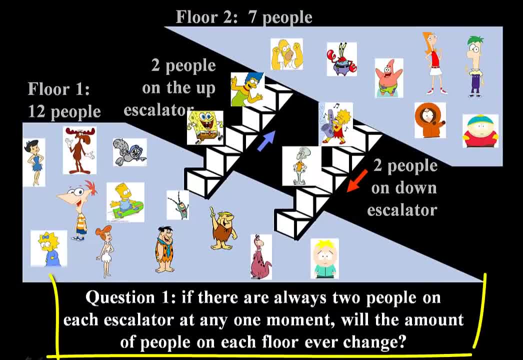 If this is our scenario, and there are always two people on each escalator at any one moment and the escalators are going at the same speed, of course, well, the amount of people on each floor ever changes. Well, the amount of people on each floor ever changes. 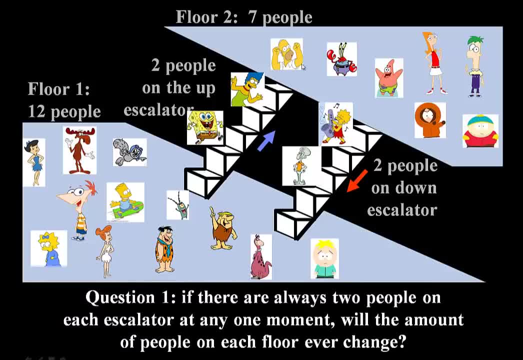 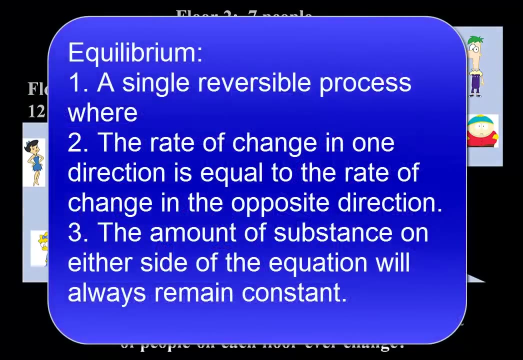 The answer would be no. as people are reaching the second floor simultaneously, that amount of people will be reaching the first floor, and so that's another hallmark of equilibrium that, because the rate of change in the opposite directions are equal, the amount of the substance on one side of the equation- in this case people- will always remain constant, and also the amount of substance- in this case people- on the other side of the equation will also remain constant. 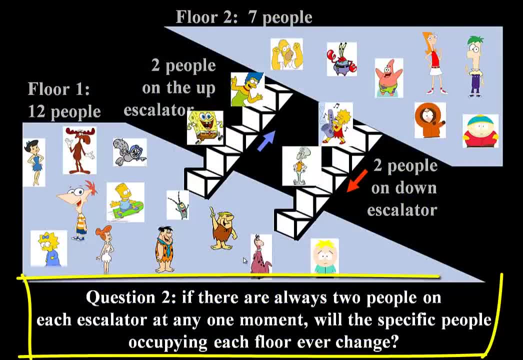 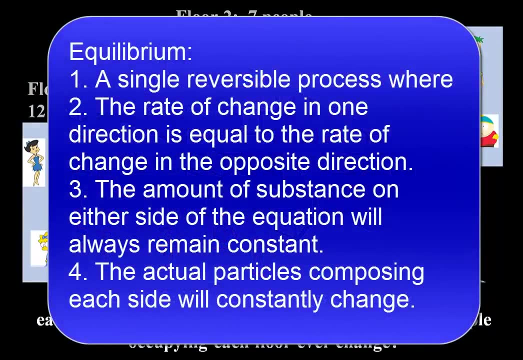 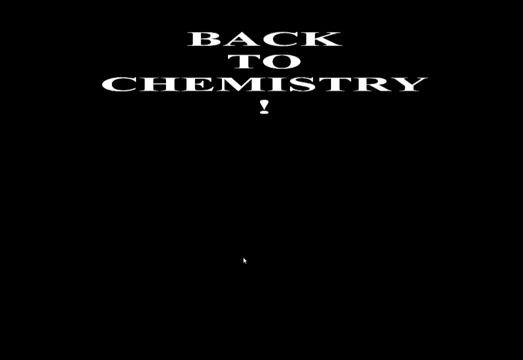 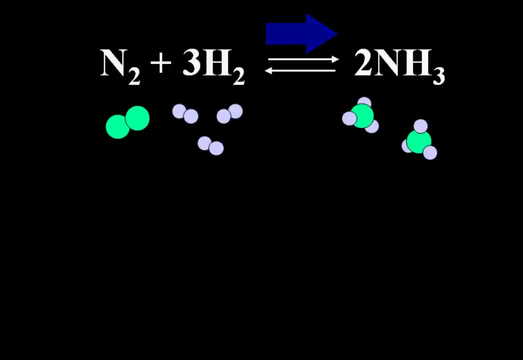 See how that metaphor applies to chemistry. a chemical reaction. We've got nitrogen reacting with hydrogen and that gives us NH3 Ammonia. If we look at what's happening, we have nitrogen and hydrogen reacting to form ammonia, while simultaneously ammonia is reacting with itself to form nitrogen and hydrogen. 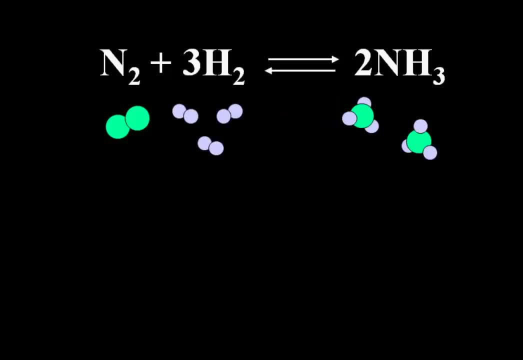 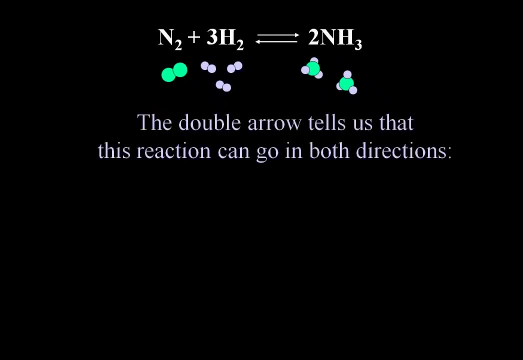 A single process that is going in two opposite directions, and if the opposite directions are happening at the same rate, that would be a chemical equilibrium. Let's take a look at how that might actually happen. So the double arrow tells us that the reaction can go in both directions. 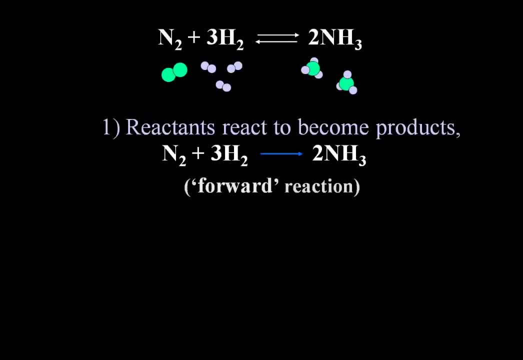 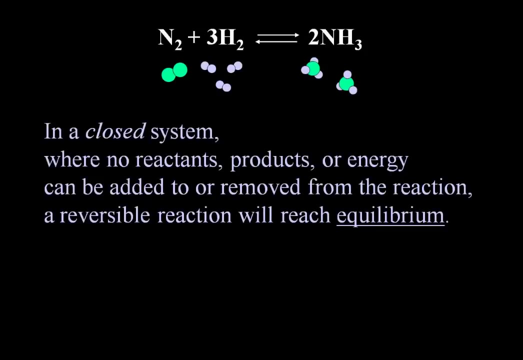 The reactants react to become products, and that's called the forward reaction, and simultaneously products react to become reactants, and that would be called the reverse reaction. So in a closed system where no reactants, products or energy can be added or removed from the reaction, 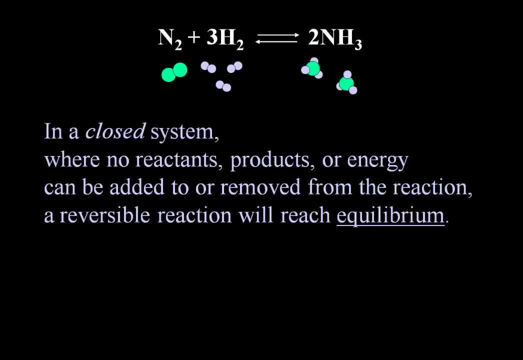 a reversible reaction will reach equilibrium. This is another very important part of equilibrium. If you're allowing reactants or products or energy or anything to disturb what is occurring in the reversible reaction, then it will not reach an equilibrium. It has to be a closed system. 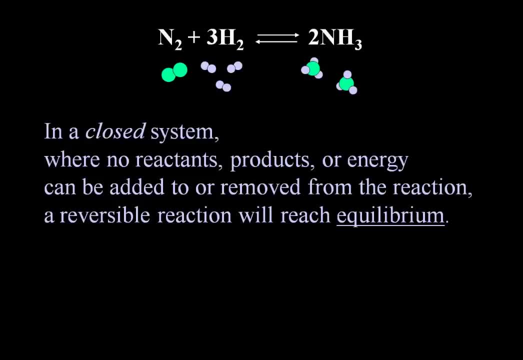 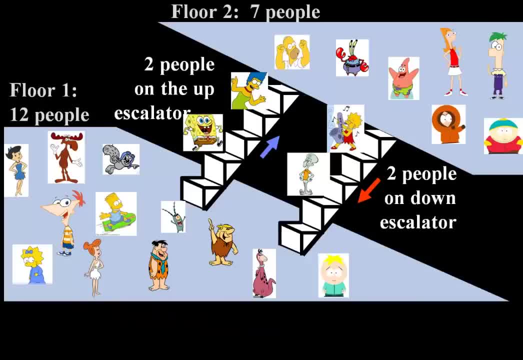 The idea of a closed system can be seen more readily because it's a closed system In the two previous examples. So here in our store there's a total of 23 people. Let's say the store owner decides to open the doors, then suddenly more people will come in. 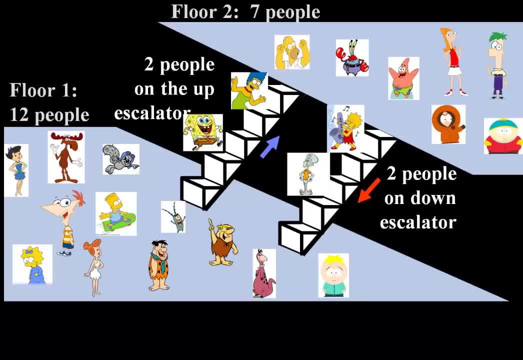 and the equilibrium will no longer exist. So it has to be a closed system. in this case, The doors of the store have to be closed after 23 people have been allowed in and eventually an equilibrium will be reached. So a glass of water at zero degrees is going to be an equilibrium. 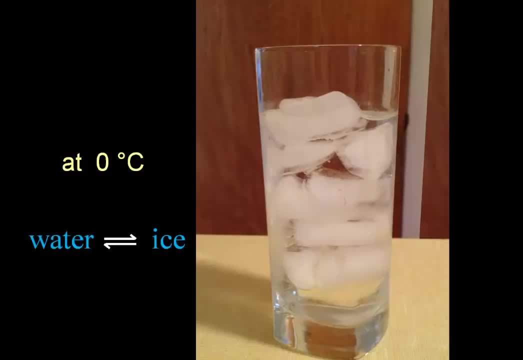 if it is exactly at zero degrees, which would allow for this equilibrium between liquid water and ice. And in fact, this is not at equilibrium because it's not a closed system. The air around the water is at room temperature, and so, therefore, we'll be constantly transferring heat to the ice. 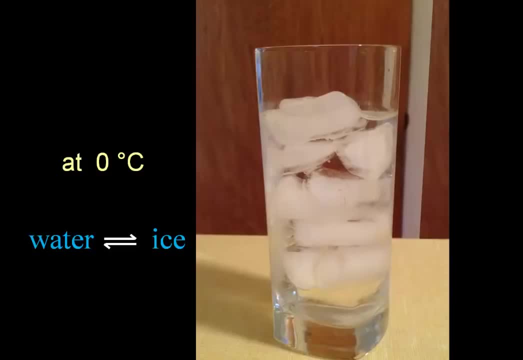 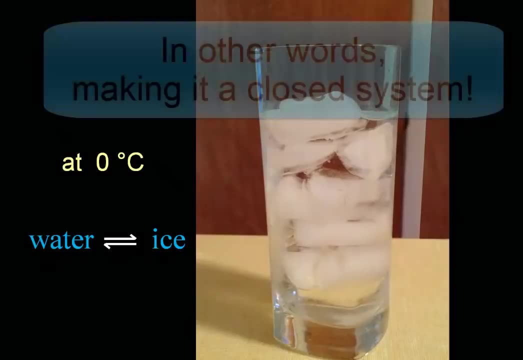 water. as you have seen in your life experience, when you put ice in water it eventually all melts And that's because it's not at equilibrium. But if we change that and isolated this so that it stayed at zero degrees, then that liquid water and ice would reach an equilibrium. There would 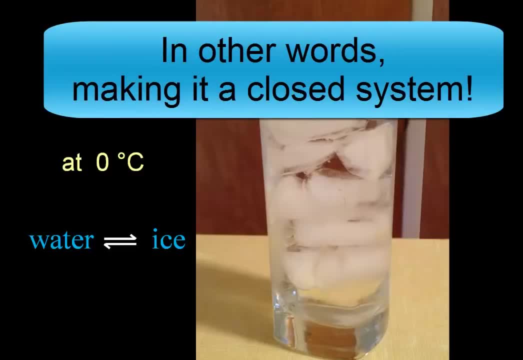 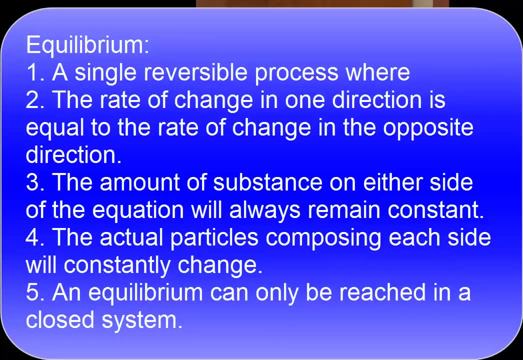 be no heat exchange between the glass of ice water and the outside, and so therefore, the rate of liquid water turning into ice would be equal to the rate of ice turning into liquid water, and it would be able to reach an equilibrium in that closed environment. 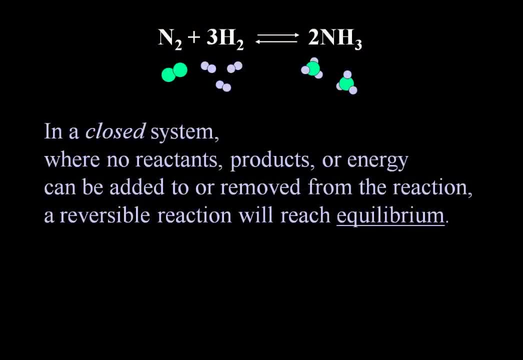 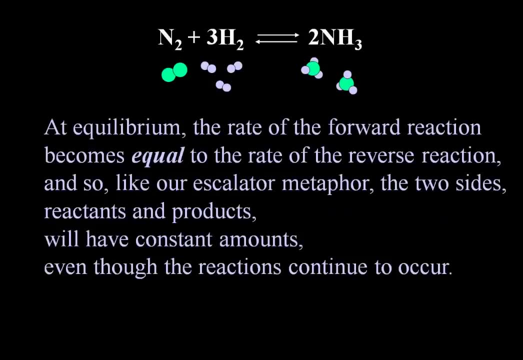 All right. so a closed system. A closed system is a very important part of an equilibrium. You can't have an equilibrium if you're not in a closed system And, as we've said before, the rate of the forward reaction becomes equal to the rate of the reverse reaction. at equilibrium, The two sides, the reactants and 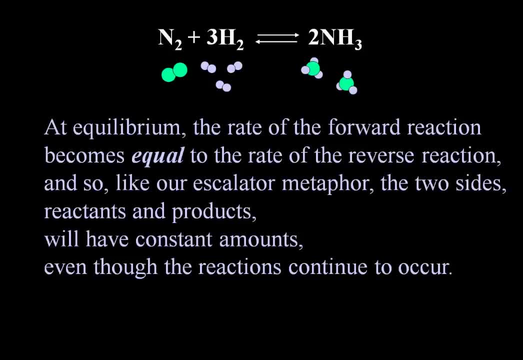 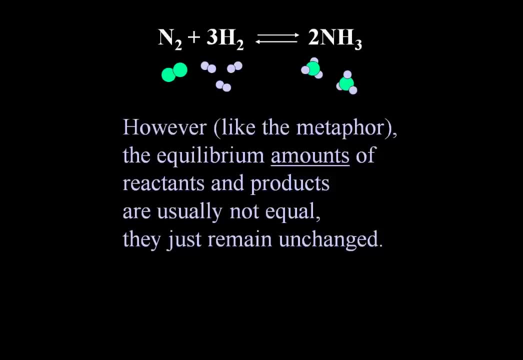 products will have constant amounts, even though the reactions continue to occur. But, like the metaphor and the ice water, the equilibrium amounts of reactants and products are usually not equal. They just remain unchanged. So, for example, in the ice water, we could have more water, less ice, or more ice, less water. 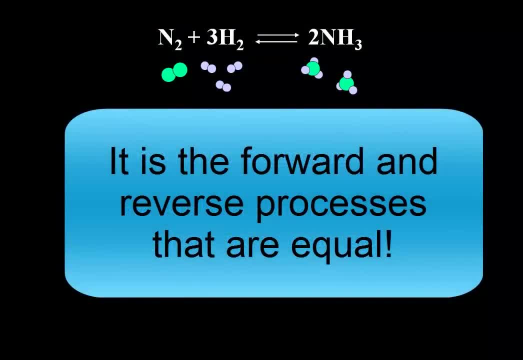 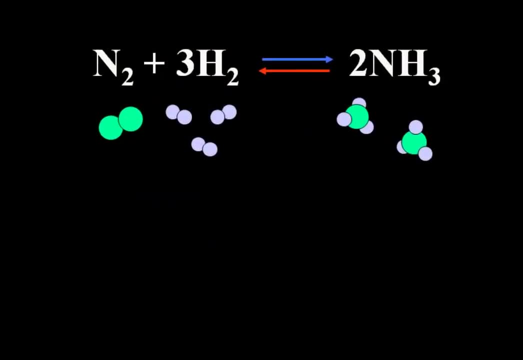 Those amounts never change. The equilibrium refers only to the rate of the forward and reverse processes being equal. So let's take a look at this from a particle perspective. Nitrogen reacting with hydrogen to produce ammonia, ammonia reacting with itself to produce hydrogen. 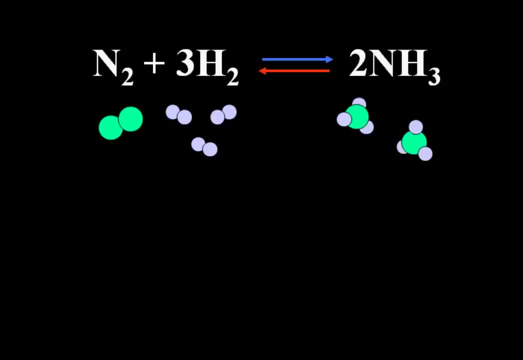 And of course we aren't just stuck with one nitrogen, three hydrogens and two ammonias, We would have many, many, many quadrillion of hydrogens. We would have millions of particles reacting in both directions. So we'll represent that with a few more. 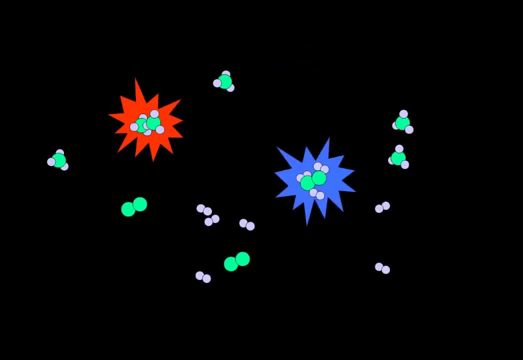 And so the particles are constantly moving. They collide with each other, And here we see that the ammonia has collided with itself, So that's going to result in a reverse reaction. And here we see that the nitrogen and hydrogen has collided, And so that's going to result in a forward reaction. 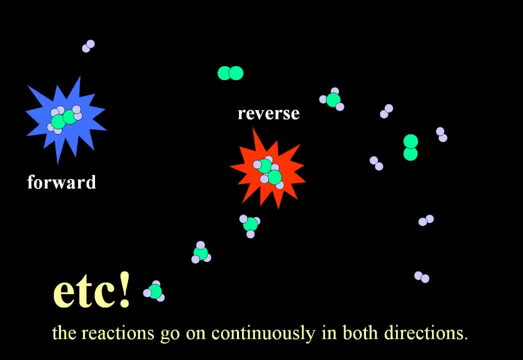 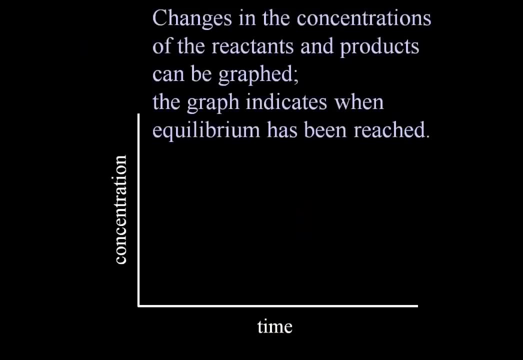 This just keeps on going. The reaction is going continuously in both directions during an equilibrium. The changes in concentrations of the reactants and products can be graphed on a concentration versus time graph, And the graph can actually indicate when an equilibrium has been reached. 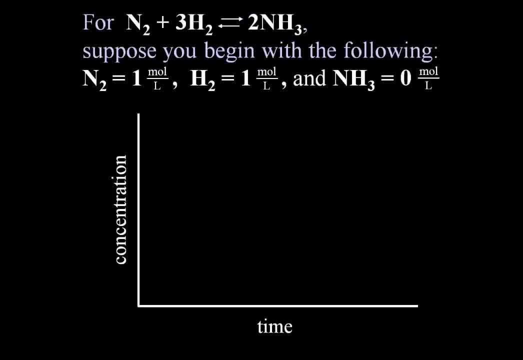 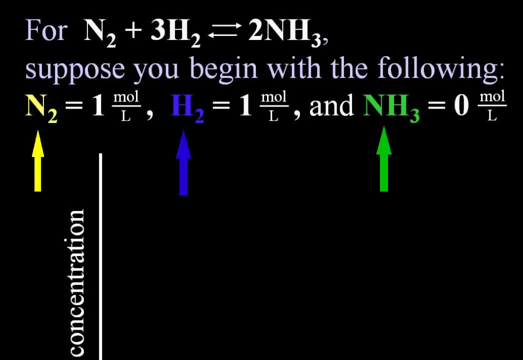 So let's take a look at that. We're going to start with only the reactants nitrogen and hydrogen, one mole per liter of each, And we're going to assume that no ammonia has been formed at the beginning of this reaction. Nitrogen is yellow, hydrogen is blue, NH3 green. 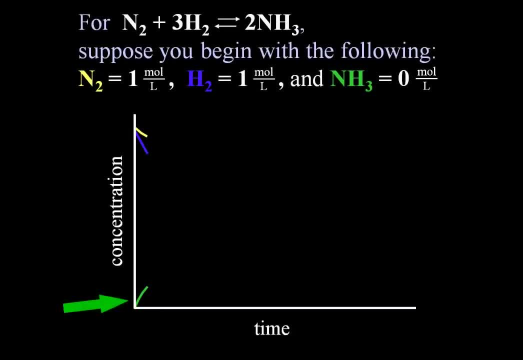 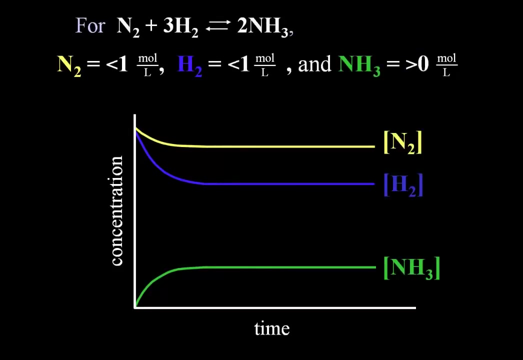 The concentration of the ammonia will immediately begin to increase as the nitrogen and hydrogen react to produce ammonia, And the nitrogen and hydrogen concentrations will immediately begin to decrease as they react and form the ammonia. But at some point they're going to reach an equilibrium. 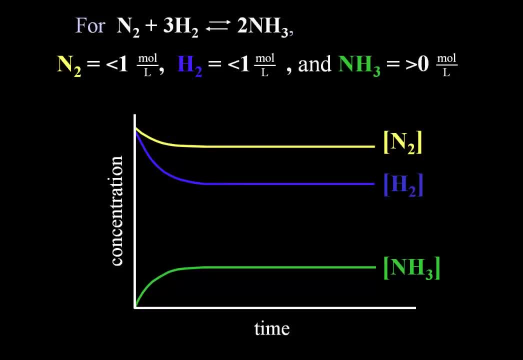 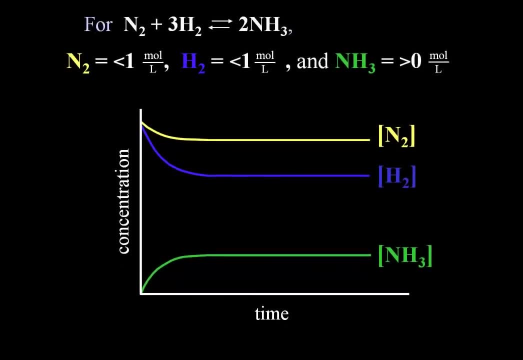 If we look on this graph and think about what we have said about what an equilibrium refers to in terms of the amounts of reactants and products at an equilibrium, at what point, would you assume by looking on this graph, would equilibrium have been established? 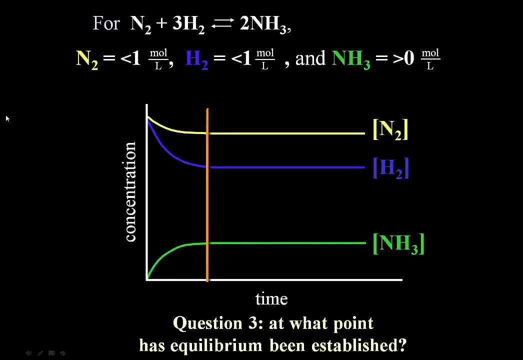 So, right here, there's no change in the amount of ammonia, There's no change in the amount of hydrogen or nitrogen, And so we can assume at that point the equilibrium has been established. The rate of the forward reaction has become equal to the rate of the reverse reaction. 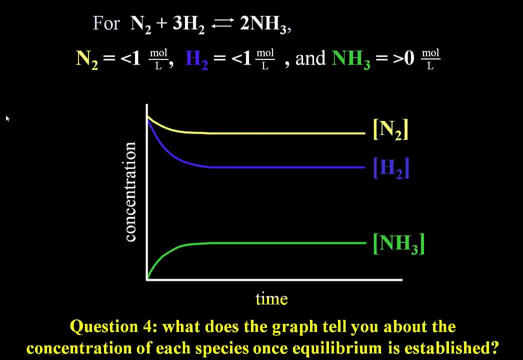 So what is the graph telling us about the concentration of each species once equilibrium has been established? Well, as we just said, if we look at this point as when equilibrium has been established, then we can assume from this graph itself that the concentration of each species remains unchanged at equilibrium. 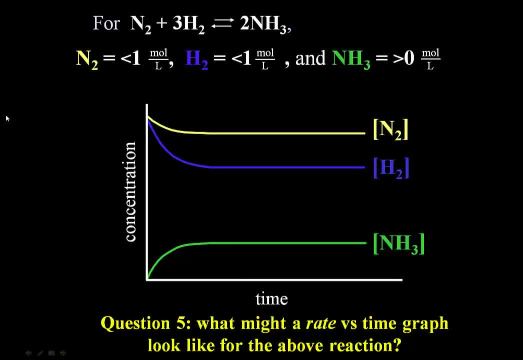 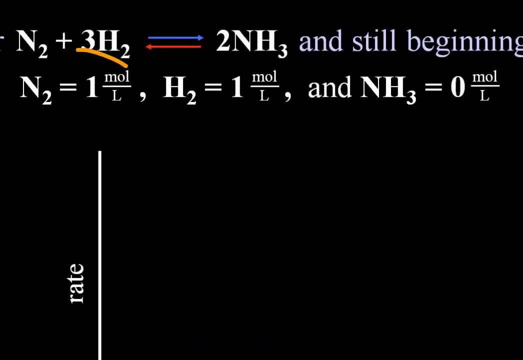 So now let's take another graphical perspective of equilibrium, and that would be a rate versus time graph. So here we have again the same reaction. We're also starting only with reactants nitrogen and hydrogen, and assuming that there's no ammonia present at the beginning of the reaction. 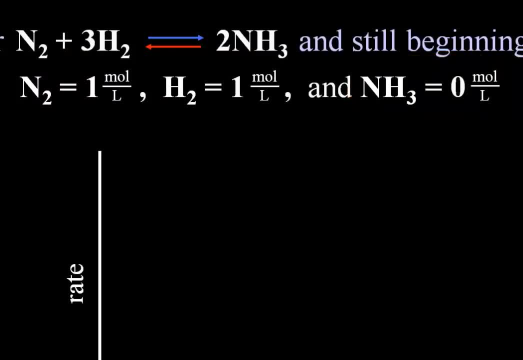 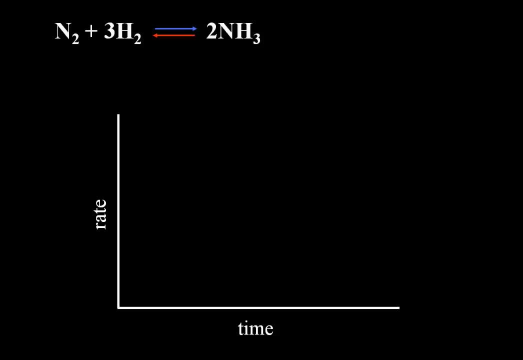 So the only thing that can react is the nitrogen and the hydrogen. As nitrogen and hydrogen react, the amount of ammonia begins to build. As the ammonia concentration builds, it reacts more and more with itself, which keeps increasing the rate of the reverse reaction. 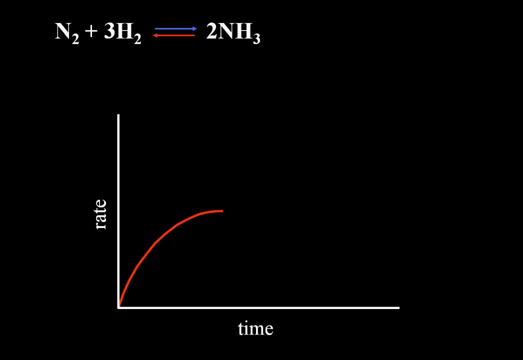 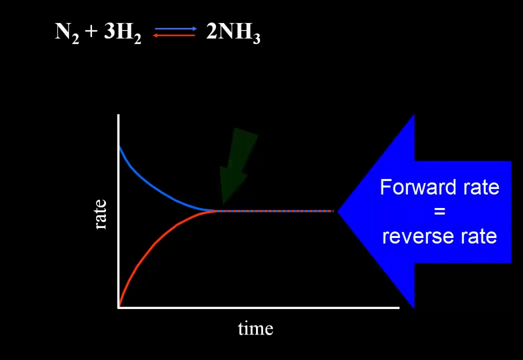 However, as the nitrogen and hydrogen react, their concentrations decrease, which in turn decreases the rate of the forward reaction. Eventually, the rate of the reverse reaction equals the rate of the reverse reaction. At that point equilibrium is established, So we can look at a rate versus time graph. 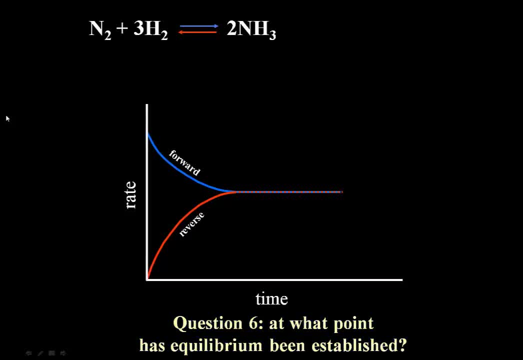 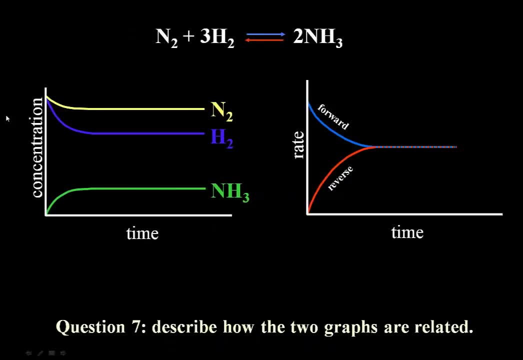 We can use this graph also to determine the point at which equilibrium is established, and that would be at this point when the rate of the forward and reverse reactions become equal. Looking at the two graphs side by side, we can see that they are related in terms of the various parameters we have established for equilibrium. 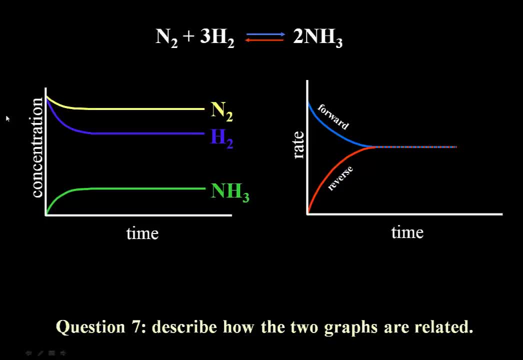 Both tell us the point in time, the x-axis, when equilibrium is established, On the left graph when the concentrations become constant, and on the right graph, when the forward and reverse rates become equal. And these are the exact same points in time for both graphs. 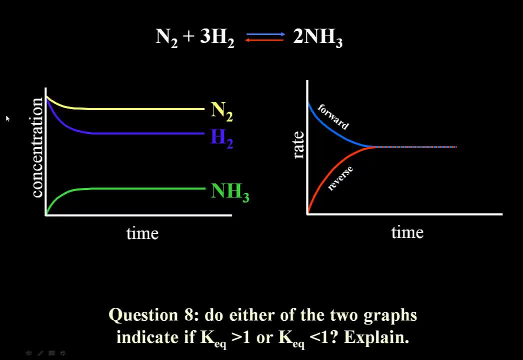 So the equilibrium constant, or Keq, is something that can also be addressed with one of these graphs, and that would be the graph on the left. The value of Keq tells us which side has more amount reactants or products at equilibrium.